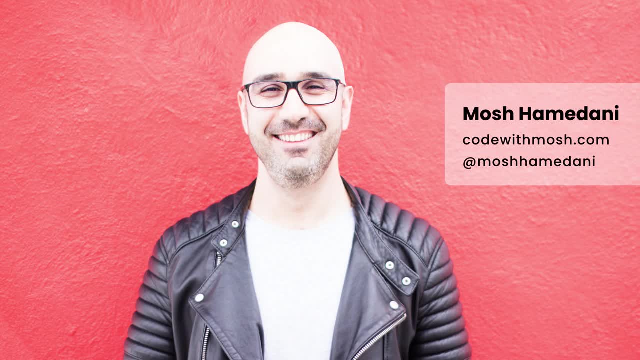 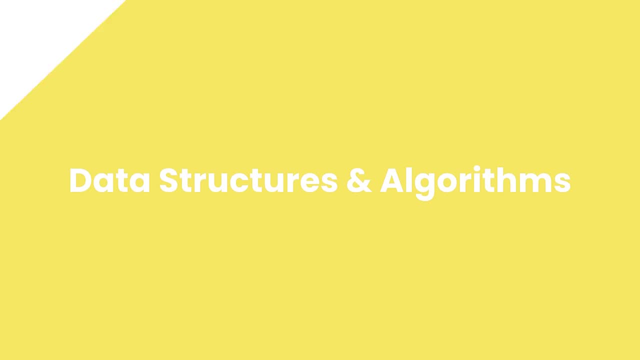 Hey guys, Mosh here. I'm super excited to announce that I just launched a new course called Data Structures and Algorithms. This is actually the first part of a series of courses on the topic. In the first part, we talk about all the linear data structures that every software developer must know. We talk about arrays. 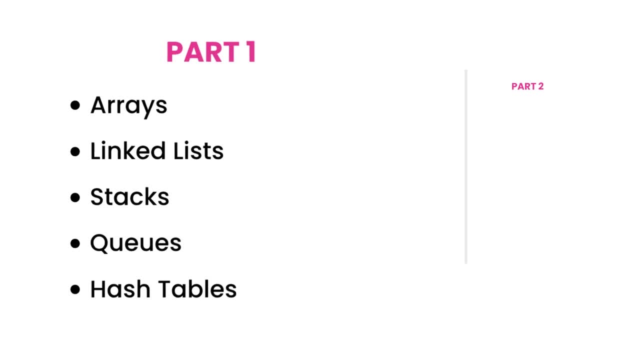 linked lists, stacks, queues and hash tables. The second part is about non-linear data structures, such as graphs and trees. I'm still working on that and will send out another announcement when it's ready. I had tons of requests for this course because data structures is one of the topics that comes up. 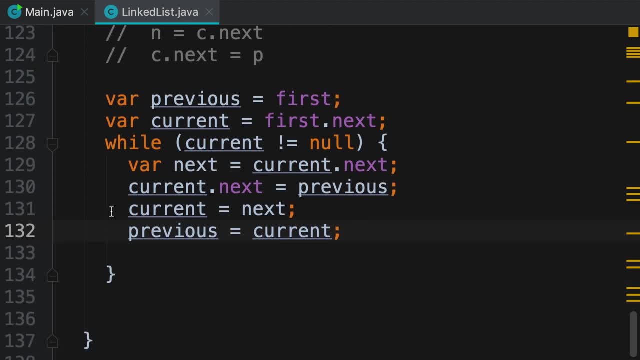 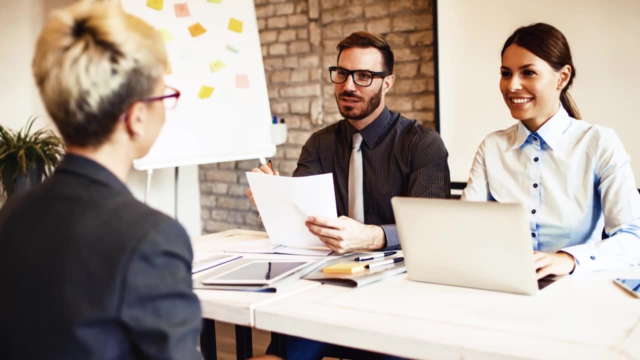 in job interviews quite a lot, especially if you're looking for a job at big companies like Microsoft, Google and Amazon. These companies always ask you questions about data structures and algorithms to see if you can think like a programmer. They don't care how many programming. 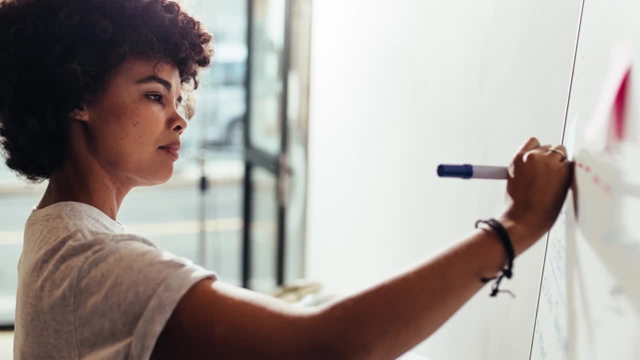 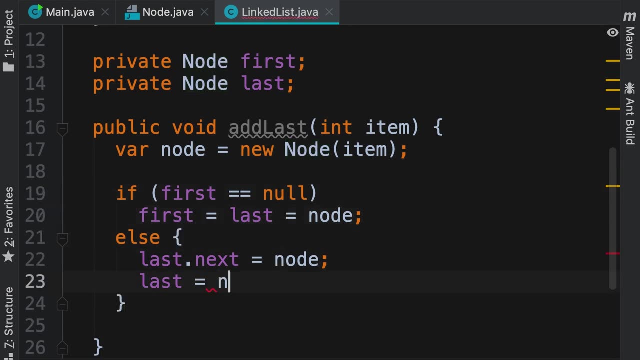 languages or frameworks you're familiar with. If you can build a website or an app but cannot solve a basic computer science problem, you're going to fail, And that's exactly why I'm going to show you how to do that. I created this course for you, to help you master this very important topic. Every single exercise. 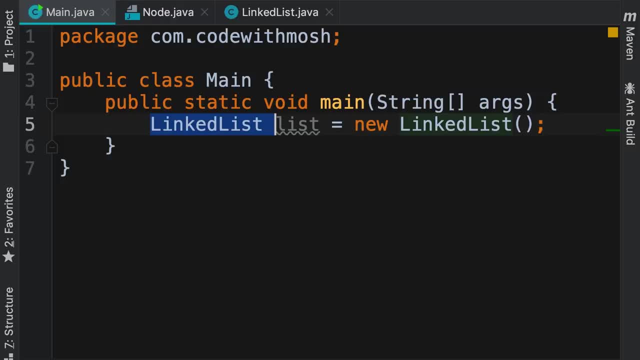 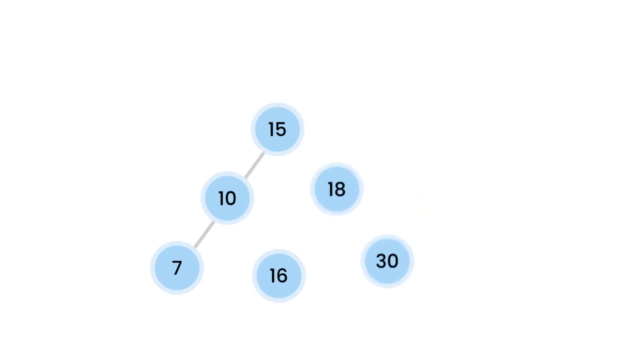 and example you see in this course is a popular interview question. I'm super excited about this course and I wish when I was learning this topic back at school, we had a course like this, Because most data structure books and courses out there are super boring and dry, Plus the code you see. 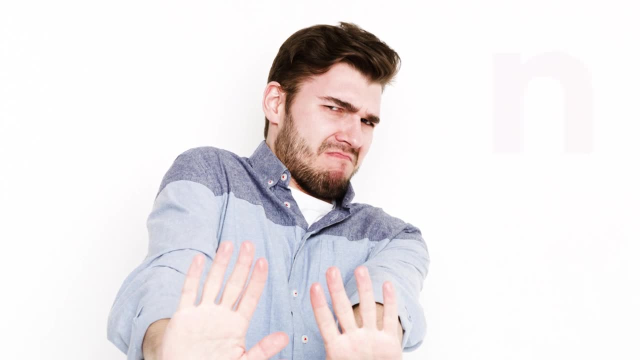 in these books look disgusting. You see a lot of mysterious variables like N, K, A and B, and you have no idea how they work. So I'm going to show you how to do that, And I'm going to show you how to. 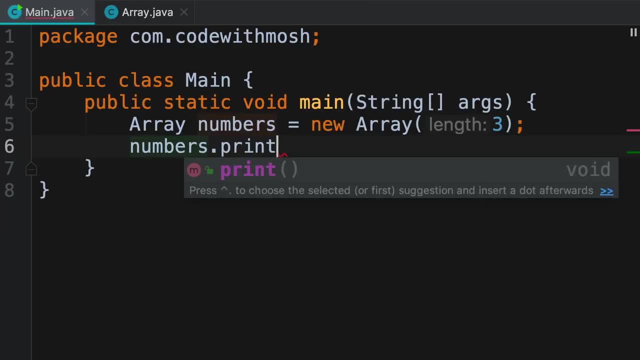 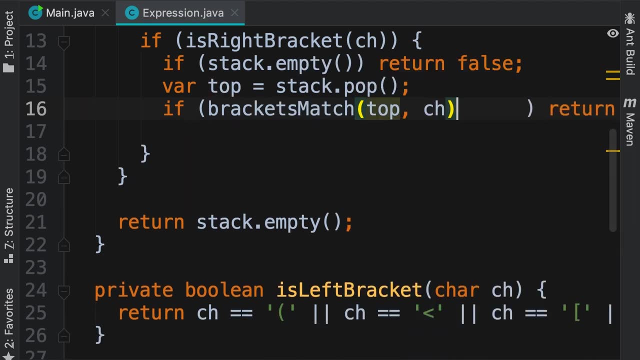 implement these algorithms work. In this course, not only will you learn everything about data structures and algorithms, but you will also learn how to implement these algorithms with beautiful code, The kind of code that can be read like a story. You will see how I start with a. 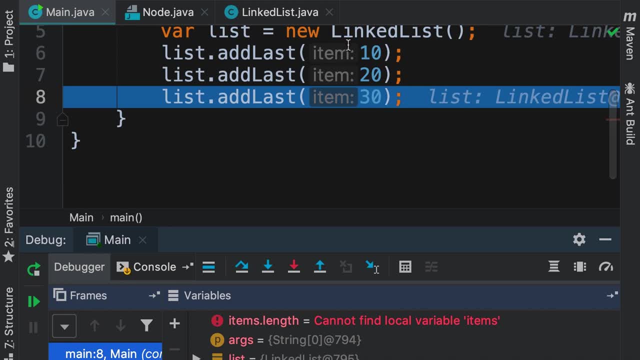 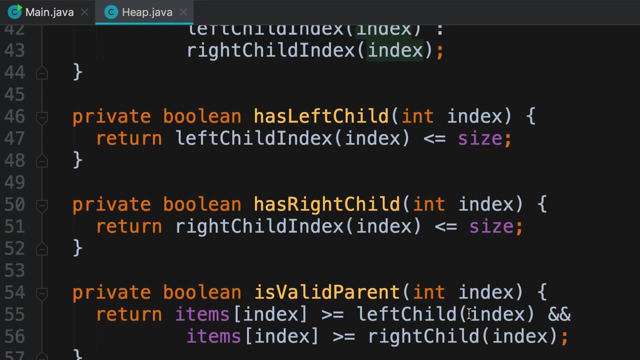 simple solution, then refactor my code and make it better and more expressive. This course is a must for any computer science students whose lecture failed to explain these topics, as well as people who want to get a software development job at a good company, Or, I would say, anyone who's.